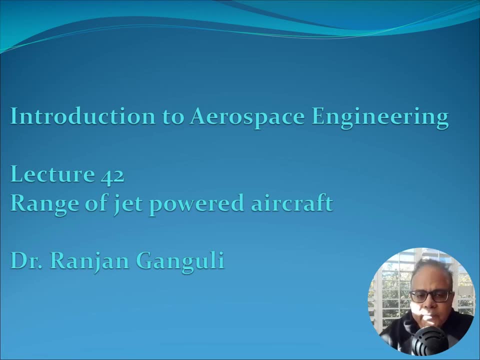 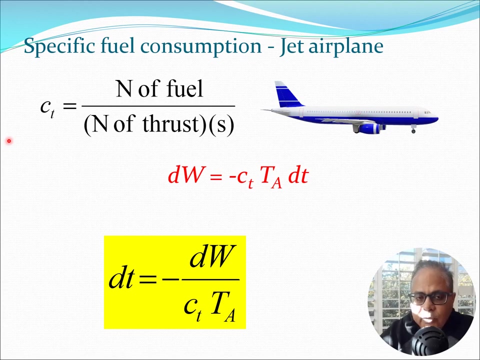 Hi students, today we start lecture 42 and today I am going to discuss the range of jet powered aircraft. I am Dr Ranjan Ganguly. Now. in the previous lecture we discussed about Ct, which is the specific fuel consumption. We will just recapitulate on that. So Ct is. 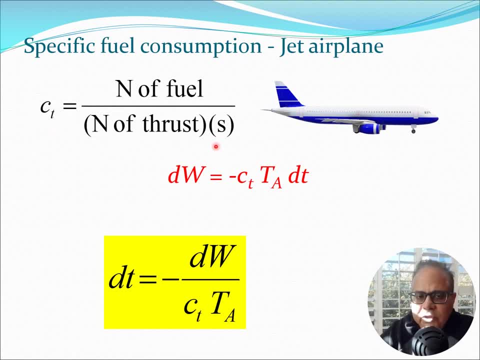 defined as Newton of fuel divided by Newton of thrust into second. So from this particular definition of the specific fuel consumption for a jet we can write this equation here. So this Ct here for jet engine is different than the C we discussed before for the propeller. 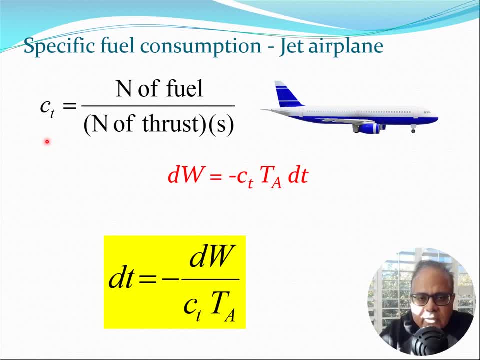 aircraft, So do keep that in mind. So what I can say is that the Newton of fuel, or the change dw, is equal to Ct into the thrust Ta into Dt. That is the equation we have written here, and the negative sign simply means that the weight of the aircraft reduces. 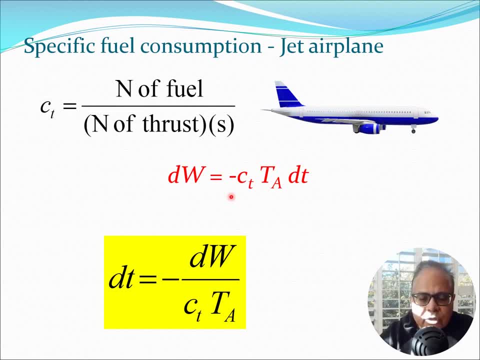 As the time elapses. So essentially, when you start the process, the start the flight, your engine or your total weight is very high and then as the fuel keeps getting expanded, the weight keeps decreasing. So that is the negative sign here, and from this equation for dw we obtain the equation for Dt. is negative dw by Ct Ta, which will let us calculate the. 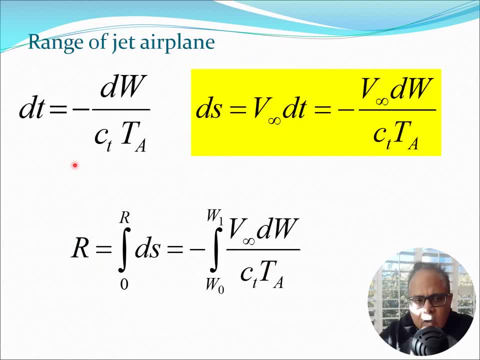 range of the jet airplane. So we get the value Dt and we multiply it by the velocity V- infinity- of the aircraft. So that gives us Ds, which is a small amount of distance which is covered in the time interval, Dt if you are flying at velocity V- infinity. So we plug in this value of Dt in this equation. 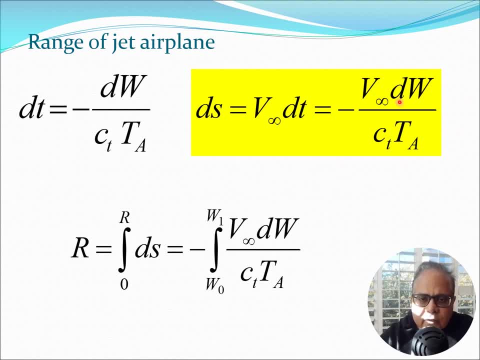 and we get this equation for Ds. So the V infinity term comes in here. Now to calculate range, I have to integrate from zero to R Ds and that gives me negative W, zero to Ds. So negative W1, V infinity, dw by Ct, Ta. So this is the general expression which I have for 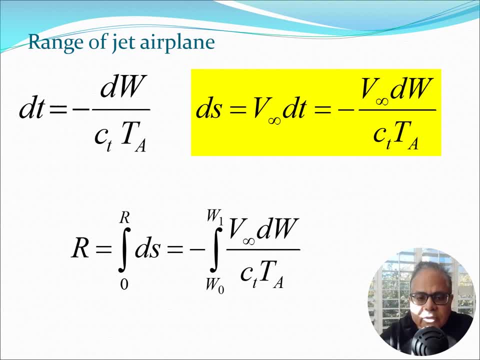 the range. and now I am going to simplify this by considering various things in steady level flight and also look at the different weights. So before we do that, let us just review the weight nomenclature. So at the beginning of the flight, let us say: you are starting from. 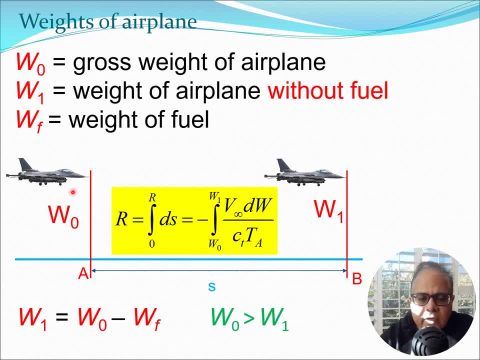 airport A and you are ending up at airport B, The weight at the beginning is W zero, which is the gross weight of the airplane, and the weight at the end of flight is W1, which is the weight of the airplane without fuel, and the difference between W zero and W1 is given by Wf, which is 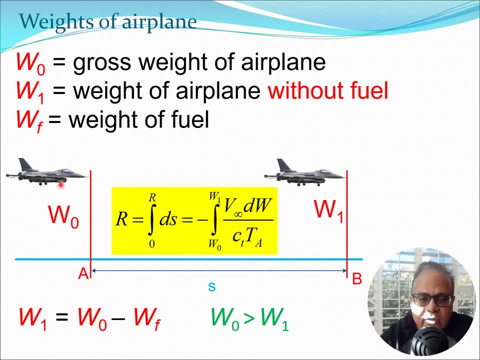 the weight of the fuel. So here the assumption is you start this aircraft with the full tank and you end the journey with an empty tank, and S is the distance which is traveled. So essentially the small increment is Ds, and when we integrate that Ds we get the range value. So this is the 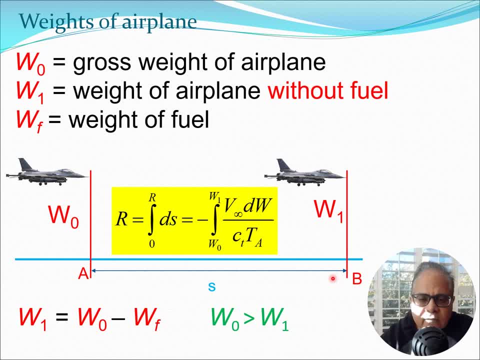 range from A to B, which is the amount of distance the aircraft covers. Now, certain points to remember here are, of course, that W1 is W0 minus Wf, and also that W0 is greater than W1 because you fly with the full tank and at the end your tank is finished. So if we want to calculate, 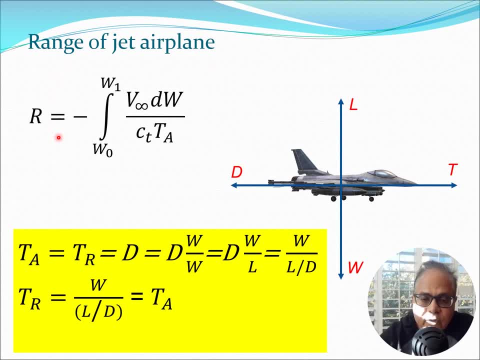 the expression for the range of jet airplane. we are going to make certain approximations and we are going to consider steady level flight. so steady level flight means that lift equals weight, trust equals drag. so i can say: ta is tr, which is the trust available, is trust required. this is ensured by the pilot. 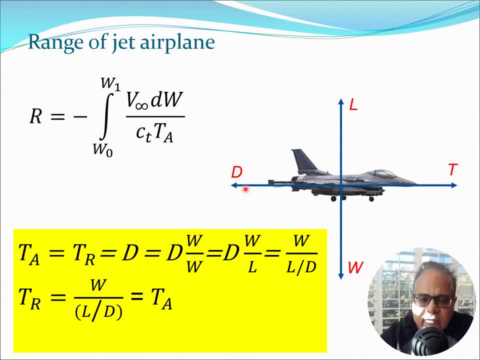 and this is also equal to drag because of steady level flight. and then i can say: drag is equal to dw by w- no problem in having numerator and denominator same here- and this is equal to d w by l. so essentially i am using the fact that weight is equal to lift. so i am putting it in. 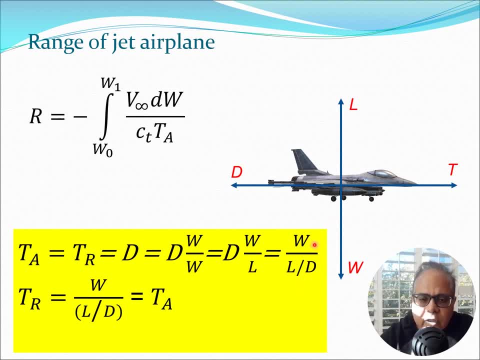 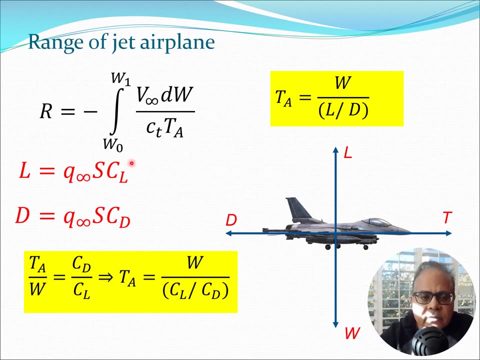 this form, then i put this as l by d and i keep w here. so this essentially lets me have this equation that tr equals w by l by d and this is equal to ta. now we are going to do some further simplifications here. we take this equation for range. 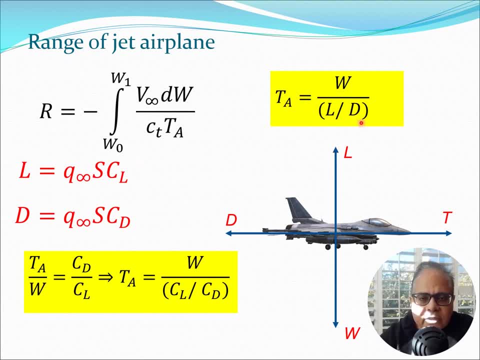 we already know, ta is w, you, you by l, by d, and do recall that l and d can be written in terms of the lift coefficient cl and the drag coefficient cd respectively. so here, q- infinity is the dynamic pressure, s is the area of the wing, and cl and cd are the lift and drag coefficient. so if we substitute these two, you can: 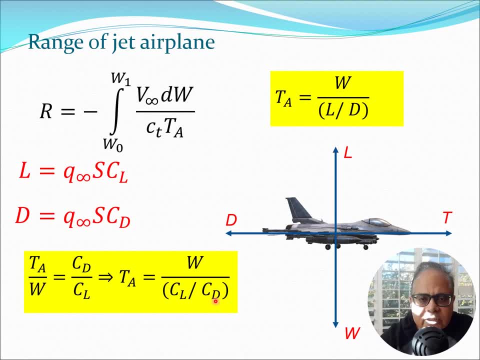 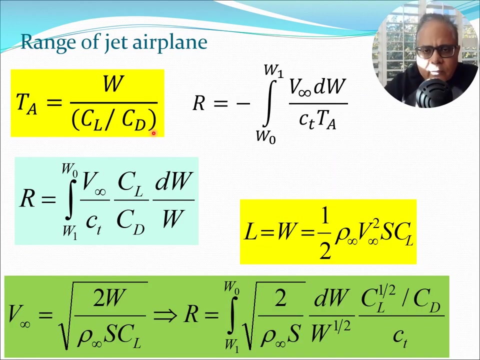 immediately see that l by d is the same as cl by cd. so essentially i can write: ta equals w by cl by cd. of course, in all these assumptions and approximations the fact that steady level flight is there is being always considered. so that's coming out from this diagram here. now we are going to work further on. 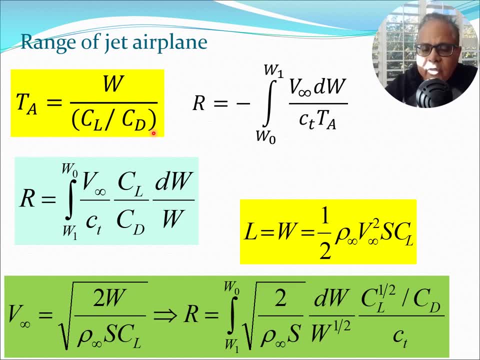 this integral to make it more amenable to closed form integration or to easy integration. so we take this expression for ta and we substitute it in the range integral, and we also change the bounds of this integral to the range integral and we substitute it in the range integral and we also. 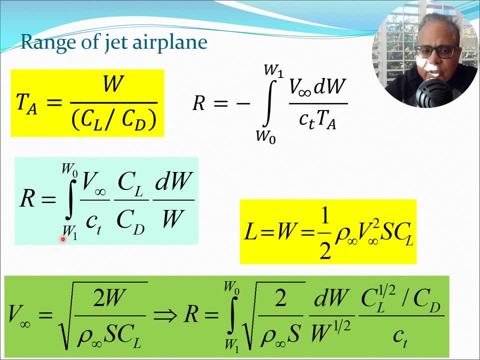 here i had w0 and w1, so i change it so that w1 goes down, w0 goes up. now i can do this, provided i change the sign, so the sign negative is absorbed here, and so the integral is flipped in terms of the bounds. now what i have here are v, infinity, ct, cl by cd, which comes from the ta term, and dw by 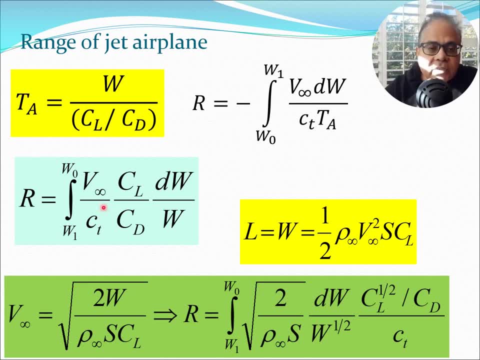 w. now there's one more problem i need to fix, and that is: what is v infinity? so v infinity can be obtained from lift, which is equal to weight, because i'm in steady level flight, and so i can write this as half: rho infinity v infinity square scl. remember rho infinity density v infinity speed. 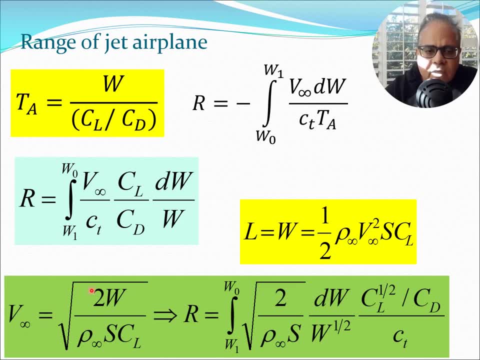 of the aircraft. now from this equation i can write v infinity also in terms of weight, and when i do that i can substitute this v infinity in the range equation and then i get this equation here so you can clearly see that that root 2 by rho infinity s. 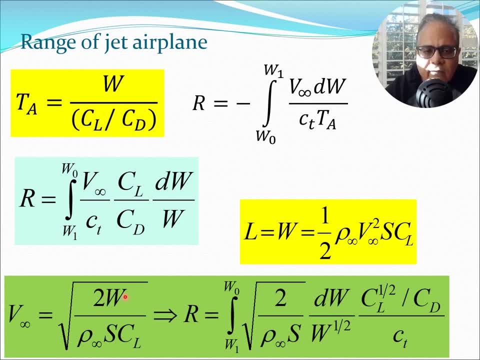 term comes from v- infinity. that is a w half here and there is a cancellation. so there is a w half produced in the denominator from the weights and so on. and there is a cl half here, or cl root, and that cancels with cl here. so a cl half term is produced in the numerator here of this range. 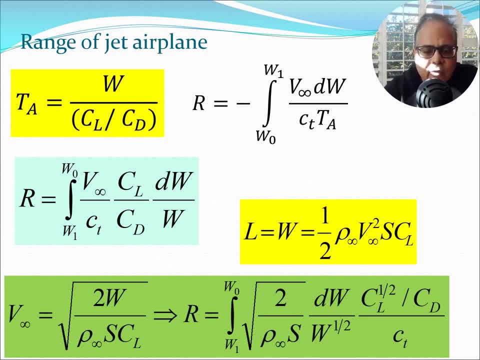 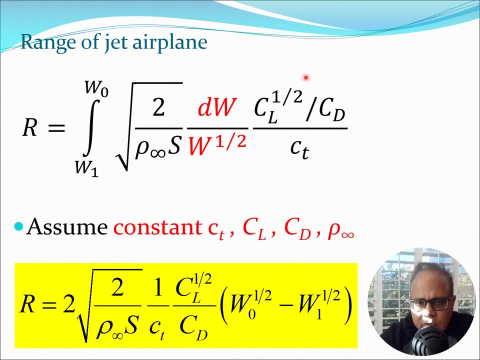 equation. so this equation is something now we are going to try to use for our further simplifications. so now let's take a good look at this equation. we clearly see that the w terms are in red here and the remaining terms are here in terms of rho, infinity s, cl, cd and ct. now, if i want this, 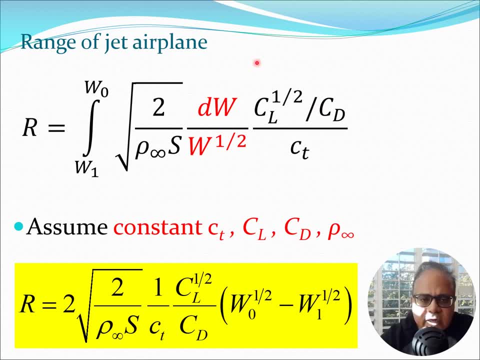 integral to be amenable to close form solution. i can extract all these things out of the integral, provided i assume these are all constant. so let's assume that ct is a constant, cl is a constant, cd is constant and rho infinity is constant, and after that i get this integral and i get this: 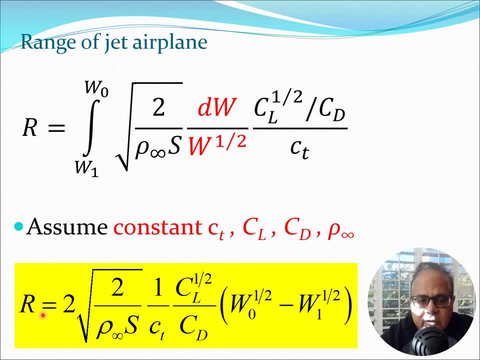 nice looking integral here, or rather the solution of this integral here. so remember that w half, if you send it up to the numerator it becomes w negative half or w minus half, and when you integrate it it becomes w minus half plus one which is w half divided by half itself. so that's. 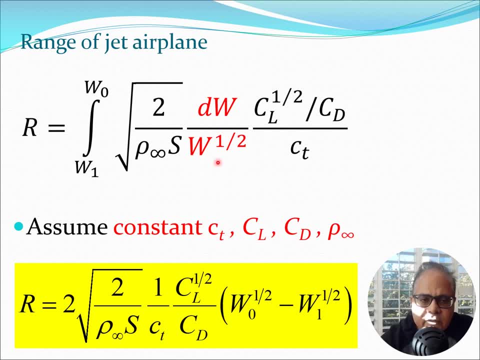 the w half term which is coming here, and the half which comes in the denominator that gets flipped and becomes a half. so that's the w half term which is coming here, and the half which comes in the denominator that gets flipped and becomes a two here. so that's the source of this two term here. so 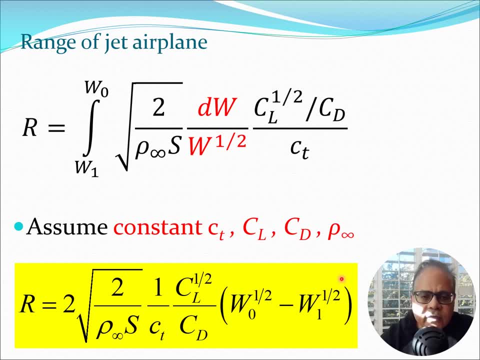 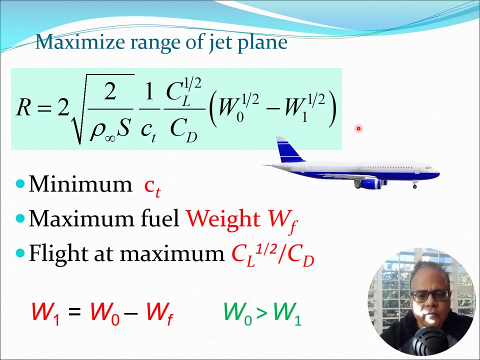 this is the integral in closed form which we get from this particular solution. so very often in mathematical modeling you do assume sometime certain things and get close form solutions, because the closed form solution does give you a lot of insight into the physics of the problem. so now let's take a good look at this equation and let's think about how we could maximize range of. 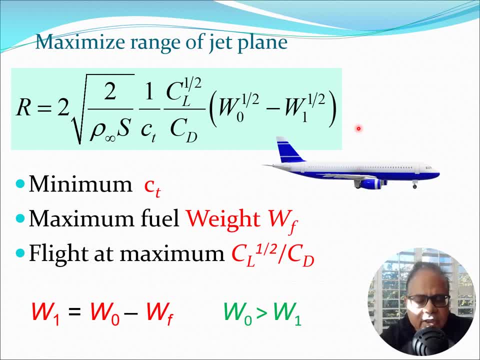 the jet airplane. now, this is a very important part of the problem, so let's take a good look at this. so let's take a good look at this. it's a very important problem because jets often travel between two airports. so if you are somebody who has been flying around, 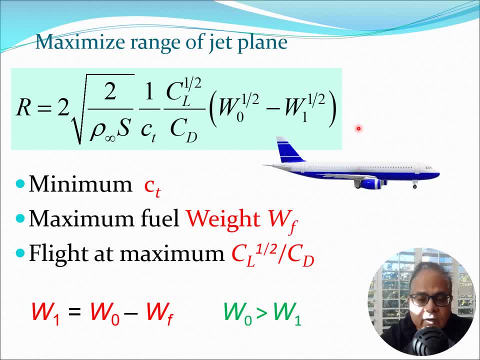 somebody who has been flying around lately, you know that if you are taking any long distance flight, for example, from London to New York, from andばं fire, from the island of Indonesia, or and ه little new york, our Tokyo to canto, then you are going to travel in one of these jet airplanes. it's very unlikely you. 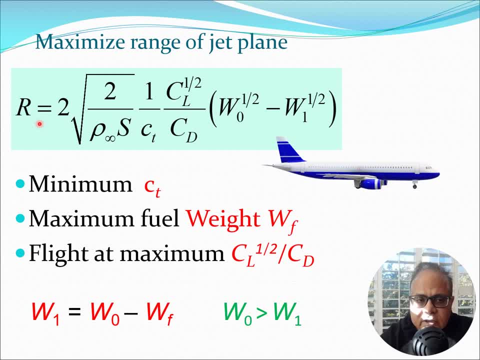 are going to travel in a propeller airplane. so if you look at this now, we will see that to maximize the cost of jet plane. so making sure this is are going to travel in one of these jet airplanes, it's very unlikely you are going to travel in a propeller airplane. so if you 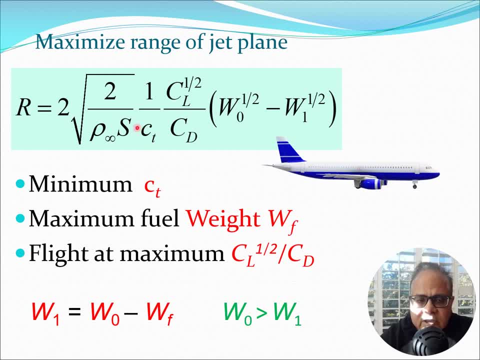 r. what we can do is we can minimize ct, which is the specific fuel consumption corresponding to the jet. we can have maximum value of the weight. we can also fly at maximum cl half by cd. so that's the value coming from here. so essentially that's something which you need to keep in mind now. if 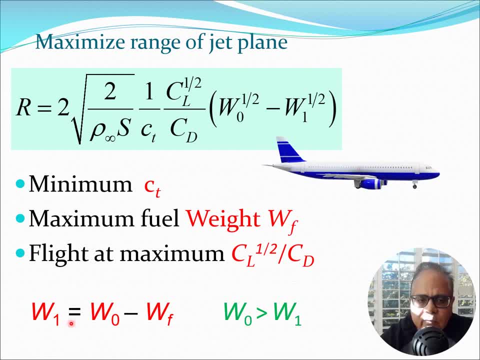 you look at this weight part, you can clearly see that w1 is w0 minus wf, so w0 is greater than w1. so this is going to be greater than w1. so essentially you want the fuel weight to be high so that w1 is relatively low, and so that's going to happen here if you have a high fuel weight of. 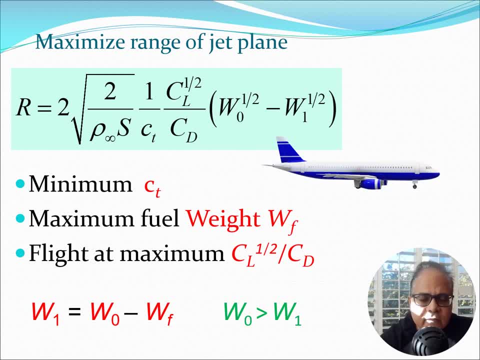 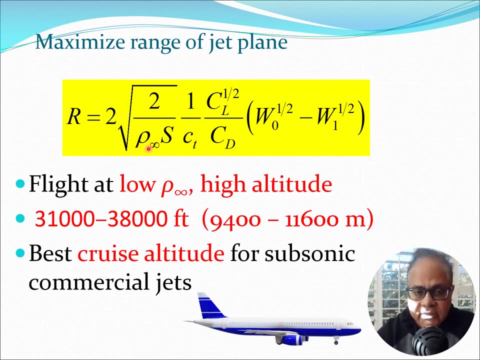 course you cannot have too much fuel weight, because the fuel tank itself is something which has to be designed keeping in mind the aircraft itself, the payload and so on, the structural characteristics etc. so one more interesting thing you will can see here is that density is there in the denominator here, which means that you want to. 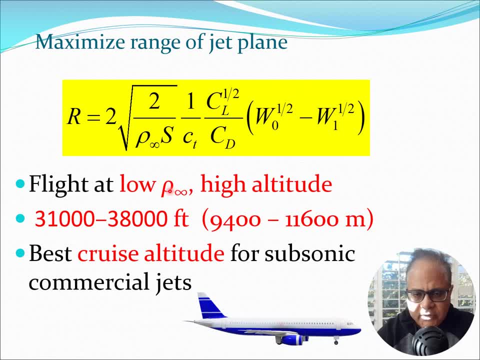 fly this aircraft at low density, so low density is going to take place at high altitude. so you typically see the jet transports. if you fly them, they travel at a height of 31 000 to 38 000 feet above sea level, or about 10 000 meters in this case. so this is a very high level if you are. 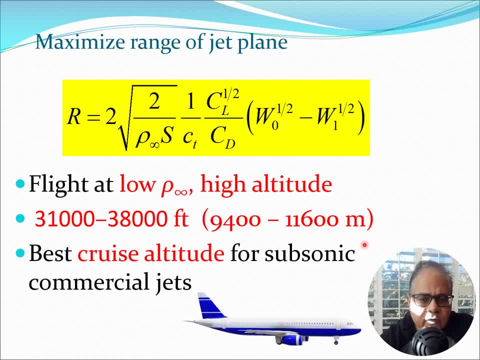 thinking in terms of kilometers. this is about 10 kilometers from the earth's surface, and the reason you do that is that density is less here. now, if you fly higher than that, some of these equations are not going to be valid, so keep that in mind. this is the density range where things are the best as far as cruise. 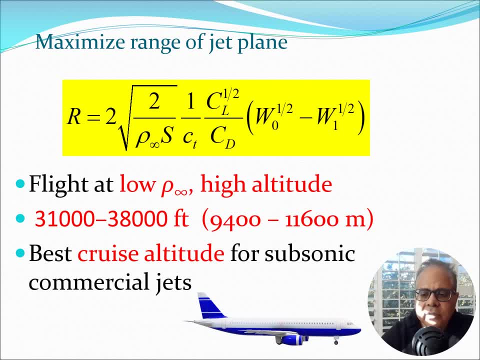 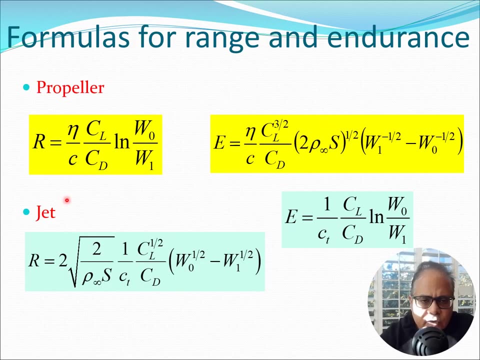 flight for subsonic commercial jets are concerned. so what happens? the airplane quickly tries to fly up to that level and then it hangs around there and near the airport where its destination is, it again starts coming down. so now we have got most of the equations for this class. we have. 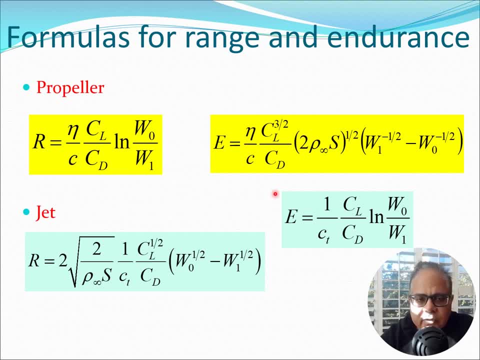 derived expressions for the range of propeller, the endurance of propeller, the range of jet and the endurance of jet, and you can see these equations are quite different. specifically, where these aircraft are often used is that very high range situations you would often prefer a jet and in 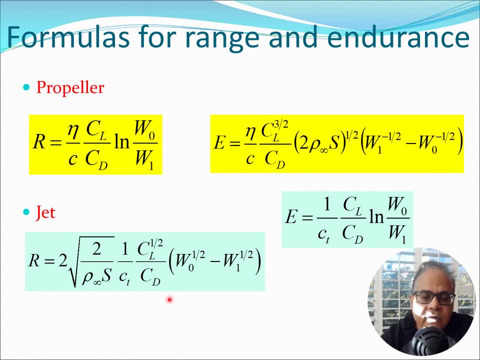 that case you would have to look at these different factors and you would have to look at the propellers. for example, you want to fly as high as possible, for a row infinity to be as low as possible. you also want to fly at the value where cl half by cd is a maximum and of course, you need 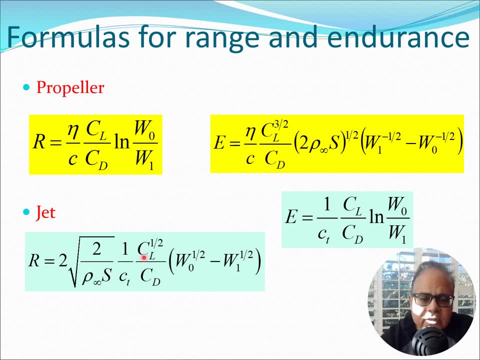 to work a lot on ct so you want to make ct as low as possible. so that has something to do with the engine systems and so on. so many a time the range of the propeller or the range of the jet airplane is very important for propellers also. things are very important because 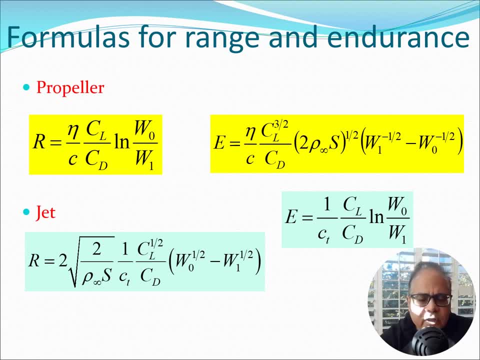 do remember that there are a plethora of aircraft out there which are propellers and in fact, if you look at most of the small aircraft where most of the pilot training takes place, you are going to see that these are essentially propeller aircraft. so very often we think that the aircraft are all. 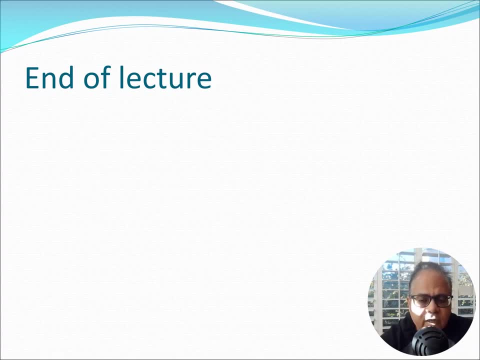 jet aircraft, because when we are flying between two cities, we often fly in jets. but what happens is that if you go to any small airport, you look at the people who train to be pilots and also people who fly for hobbies. they often use propeller aircraft and propeller aircraft are also very popular in developing. 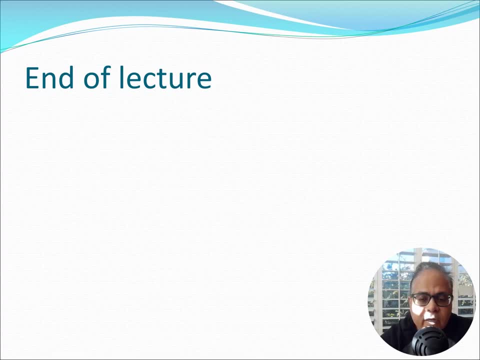 countries where the fact that they can fly from airports which are relatively small and they have runways which are relatively small is very important, and very often the cost of the propeller aircrafts are also quite less. so many a time propeller aircraft are being widely used and in 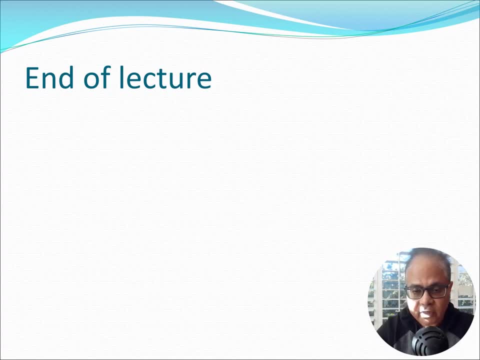 fact, there are a very large number of small propeller aircraft which are flying around on any day around the world, so this is a very important thing to keep in mind when you are flying. so these aircraft are very important. there are a lot of small business and medium-sized businesses. 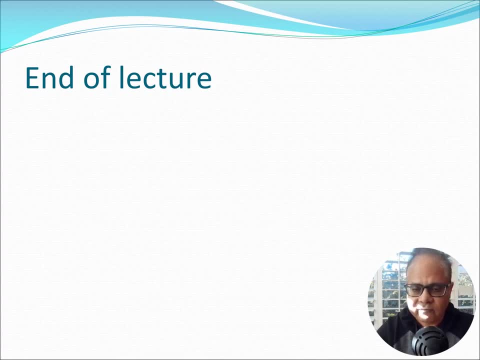 which make such propeller aircraft and it's very easy for any country or any company to make a small propeller aircraft compared to making one of the large jet aircraft, because, as far as large commercial jets are concerned, there are very few companies doing that. there is Boeing, there is Airbus and there are a few companies besides that. so that is more of a duopoly. it's very hard to break into that market. but to break into that market it's very difficult to do that. so there are a lot of small business and medium-sized businesses that are going to break into the market for smaller. 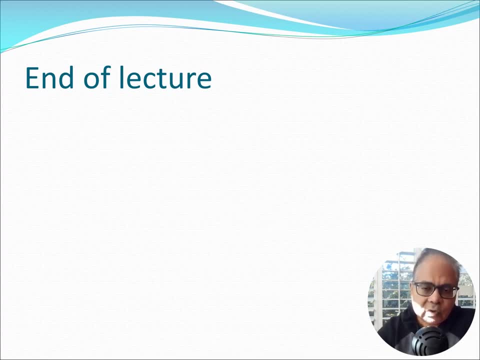 aircraft- smaller jets, smaller propeller aircraft- is much more possible. so I'll end this video here. do remember that these closed form equations are all about steady level flight. they do not include takeoff and landing. that's something we are going to study in the next few lectures, but before that, 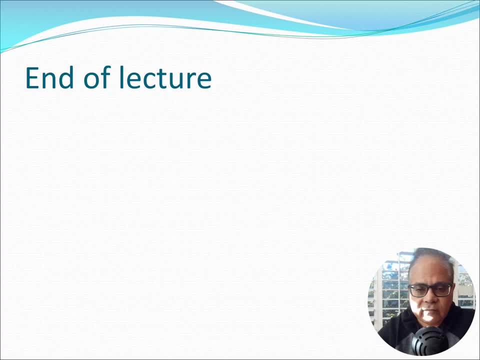 I'm going to make a lecture about the values at which you should fly this particular aircraft. so CL by CD max, CL. 3 by 2 by CD, max, CL half by CD. So all these conditions where we need to fly the aircraft to get the maximum performance.